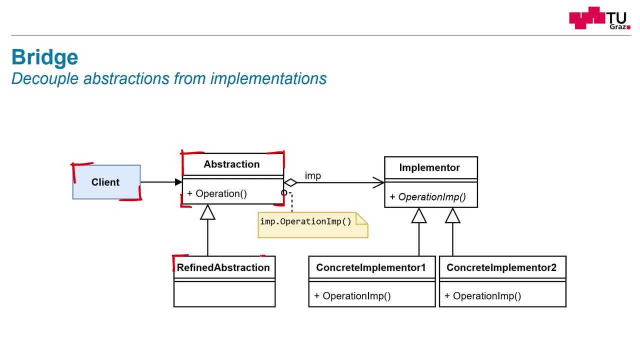 And of course, there has to be some concrete implementation for it. Think of the different graphical user interface widgets which exist for Python, for example. So here we are in user world, But all these implementations need to use some graphically basic primitives which the operating 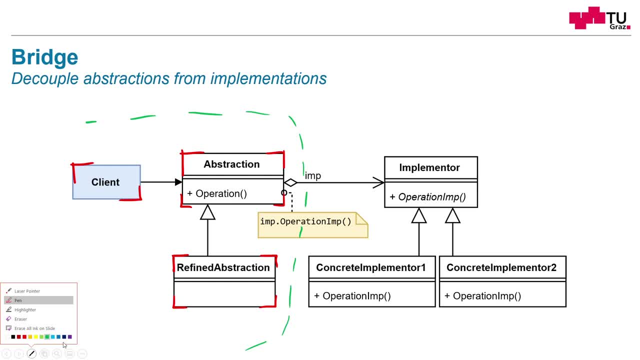 system supplies. This is a different world. So here the operating system begins And we have some graphical primitives. We can draw pixels, we can draw lines, we can draw text and so on, But there is no concrete notion of buttons. We can draw lines, we can draw text, we can draw text, we can draw. 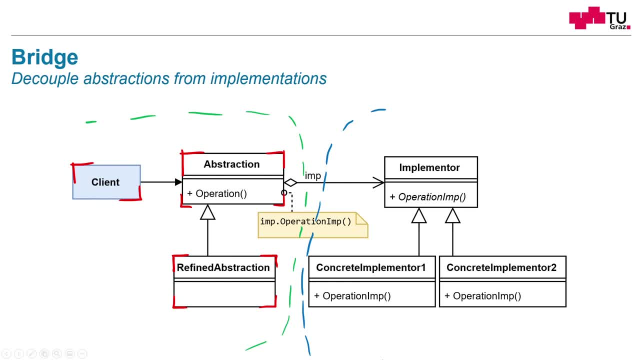 text boxes or even a window. So this is another world And in addition to this, we have these basic primitives, But depending on the installed graphical libraries, for example OpenGL or DirectX or some other graphic libraries, these can be implemented differently. For example, there could 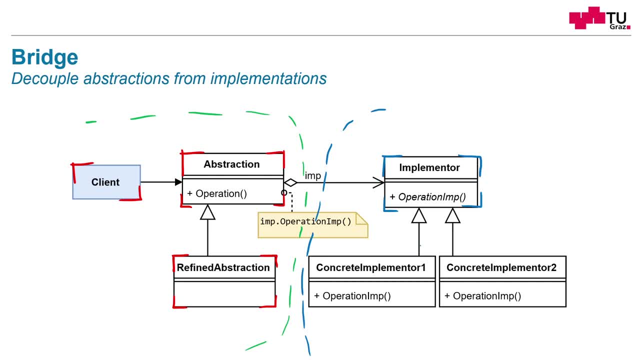 be an implementation which runs completely on the CPU or there could be an implementation which runs on the graphics card. Our implementation can be implemented on the graphics card, So we can see that the applications can be implemented differently and can evolve independently, But the abstractions here for the user, for the client, they should stay the same. For example, we don't. 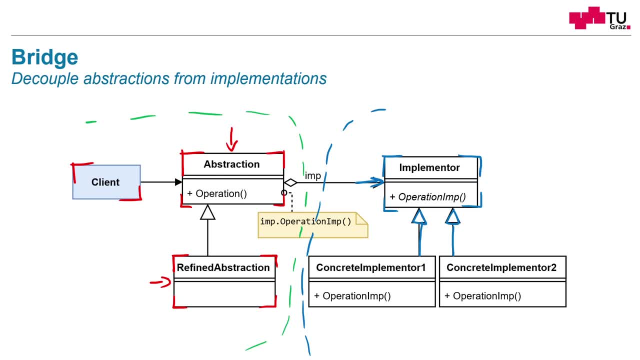 have a simple window system. Maybe we have a fancy window system where we have animations, or think of Linux, where we have different window managers and different styles which the windows can take on. This is the idea of the bridge pattern To have an implementation. 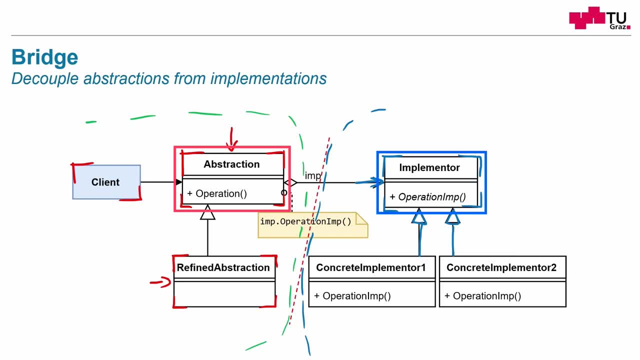 or an abstraction layer on both sides of the system, so on the implementation side and on the abstraction side. Basically, these are adapters for both sides And by doing it this way, both sides can evolve independently from each other. And you may ask: where is the bridge here? Here it is. 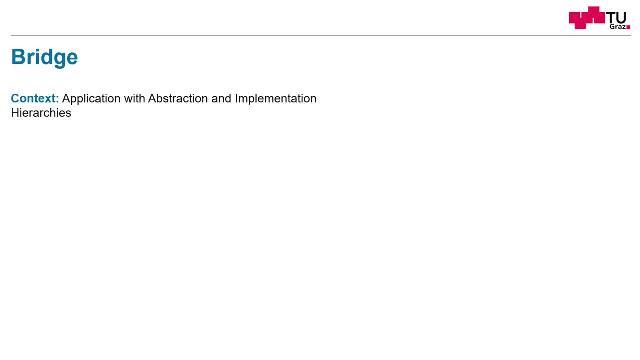 What are the properties of the bridge? The context is we have an application which has separate abstraction and implementation hierarchies. The problem is now: how can we decouple the development of both hierarchies, The forces are. we want to avoid permanent binding between. 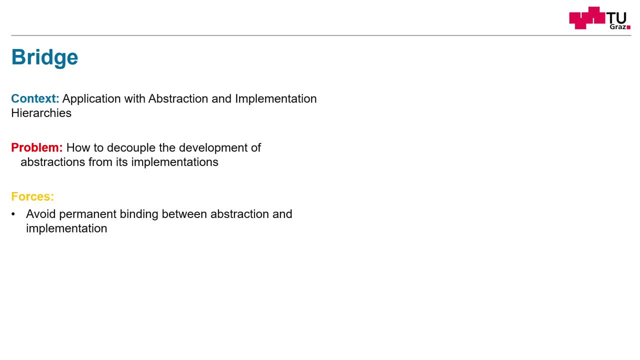 abstraction and implementation If all our window systems would be bound to the underlying graphics library, for example DirectX. whenever Microsoft comes out with a new version of DirectX, all our window systems have to be re-implemented, which is not very useful. So we can't have a single window system. 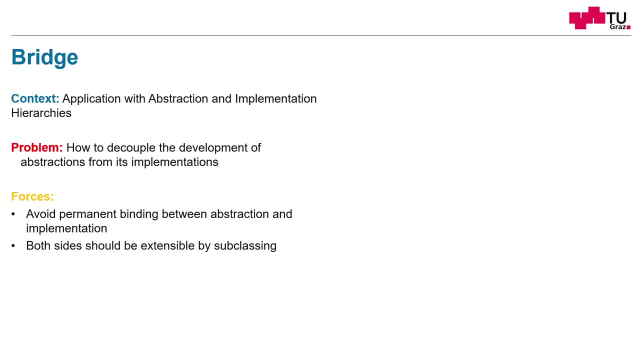 So both sides should be extensible by subclassing. For example, our window system should be extendable and our underlying graphics library should be extensible. Changes should be contained to one side, For example, if we develop a fancy animation system on our window side. 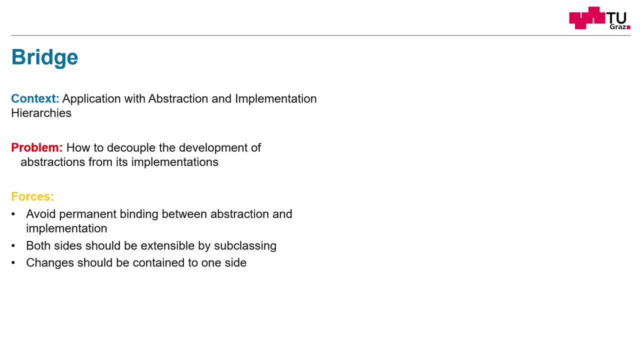 the underlying graphics library should not have to change And we want to hide the implementation side completely from the client. So the client doesn't have to implement DirectX matrices and apps in order to implement a graphical system. It just wants to use buttons, text boxes and so on. 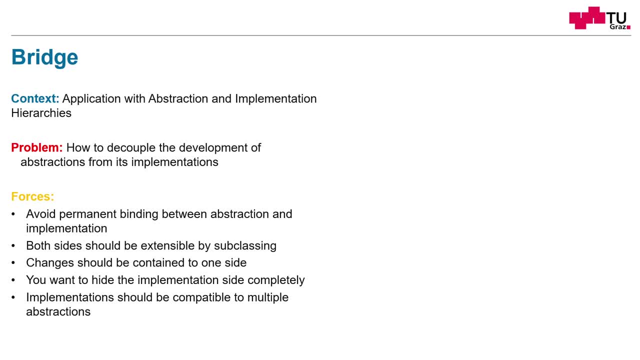 The implementation should be compatible to multiple abstractions. Especially on Linux, this is very visible If you have different window managers. they all look differently. but use the underlying graphical primitives in the background. The solution is to create two interfaces. Firstly, the implementer interface. These are the internal primitives, the basics. 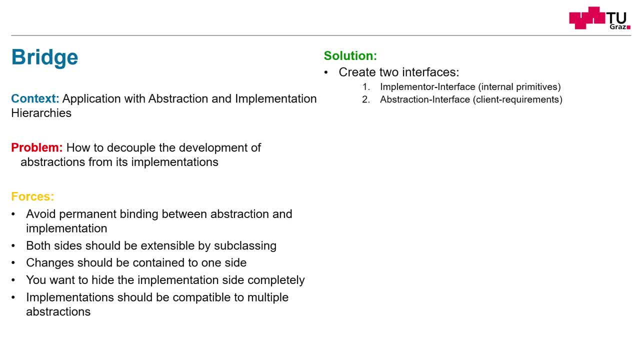 and an abstraction interface which covers the client requirements. This is actually the interface the client has to work with. Therefore it should cope for the client requirements. And then we have to implement those interfaces with individual classes. Then we can implement more than just one class We can derive. 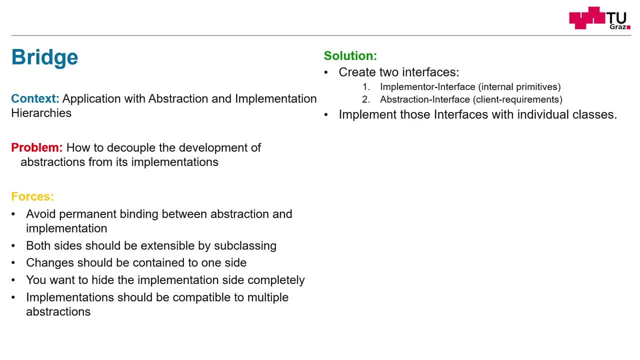 from them We can build up whole hierarchies of classes on both sides And then in the abstraction, we only are allowed to use the implementation interface. So we are not allowed to use the concrete implementation interface, We are only allowed to use the concrete implementation. 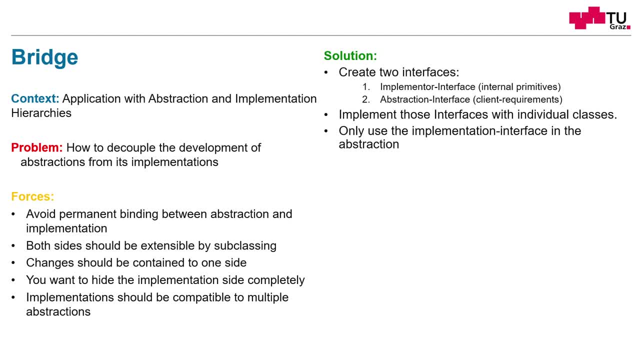 interface, just their abstract interface. And of course, the client only is allowed to use the abstraction interface. What are the consequences? We have decoupled abstraction and implementation. We improved extensibility. Both sides can grow independently. We hid away the implementation. 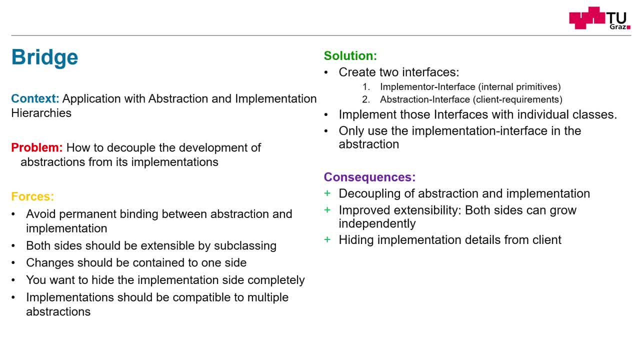 details from the client because he only uses the abstraction interface. The implementation can be configured at runtime, Or the implementation can be configured at runtime Also at compile time. we don't have dependencies on the actual implementations anymore, but just to the interfaces, which is a good thing. It encourages layering. We have at least two layers.